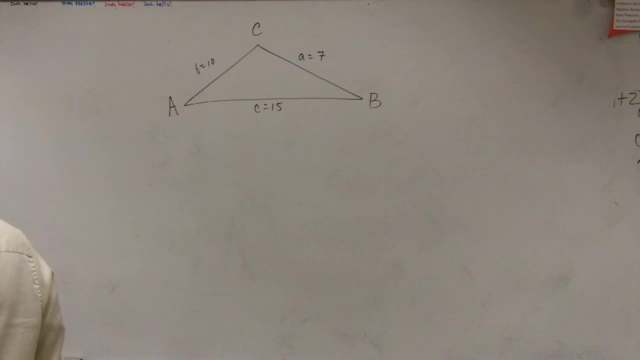 Ooh, I like it. Wow, Cool, Alright. so what I want to do is I go over how to solve or find the missing values of this triangle. So what we're given over here is we're given a triangle and we're given all the side lengths, alright, But we're not given any of the angles. So what we learned before is, obviously, you use the law of sines, And in the law of sines it was a proportion right: The side length over the sine of its opposing angle was equal to the sine of its opposing angle. 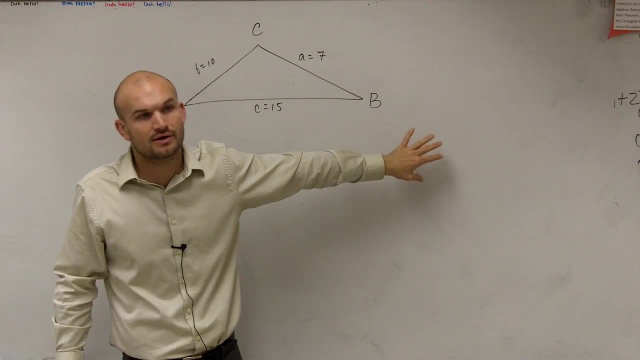 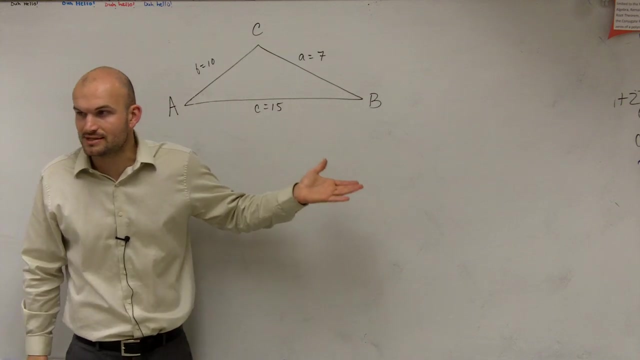 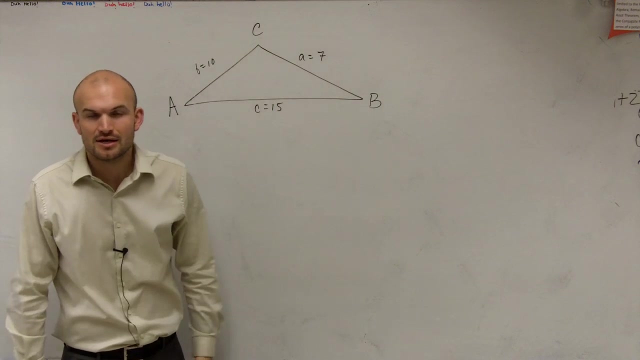 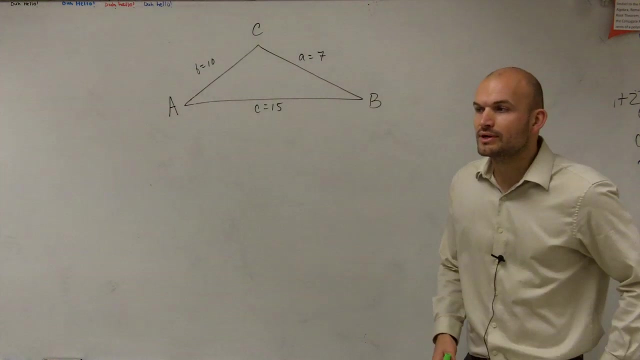 So we're given the side length of the opposing angle, of all three of the other angles right And their opposing side length, But we have a problem with this because we can't apply or use that proportion, because we don't even have a ratio that's complete right. You can't even set up a proportion that would have only one missing values because you don't have any of the angles. So to try to use this Kara for law of sines is not going to work alright. So what we're going to have to do is look into this by using the law of cosines. 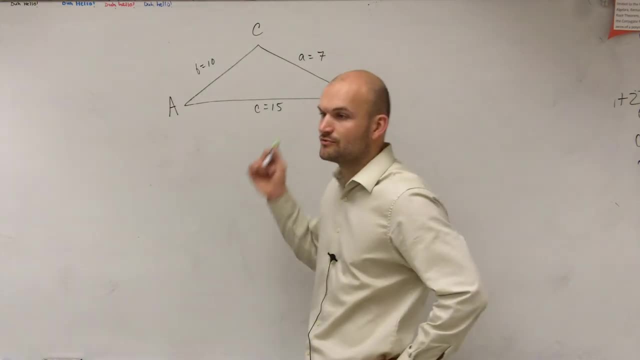 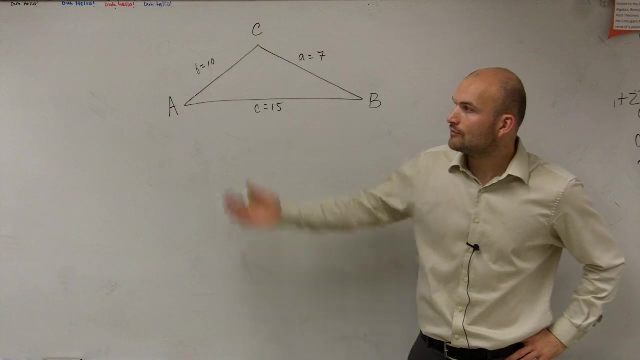 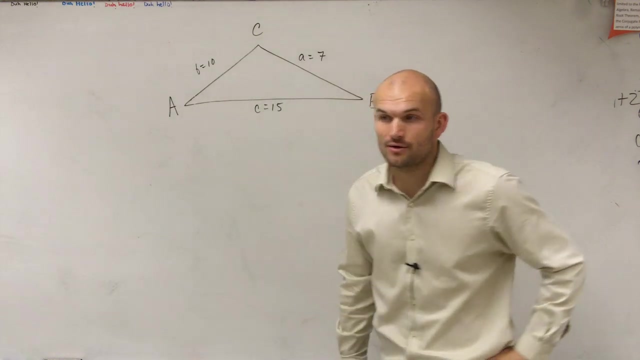 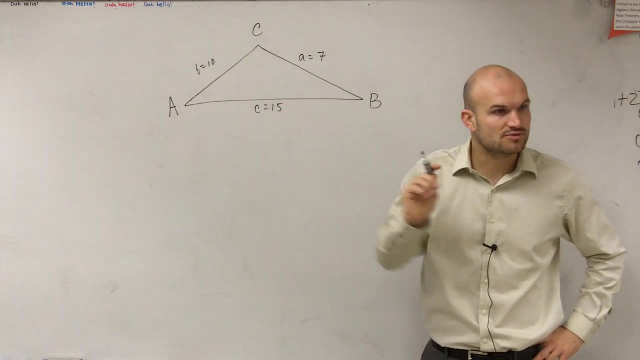 And there's a question here- There's a couple little tricks that we need to do when using the law of cosines, especially for a problem like this. You could say, well, I don't know what a, b and c are, And you can see, I wrote down the law of cosines over there. Well, for each one of those, they have a cosine of a, cosine of b or cosine of c. So you could say, well, you could just pick any one you want to and solve for that angle. But the problem that we're going to want to come up with is we don't want to arbitrarily just pick any angle. There's one angle that I want to be able to solve for first of all, And I'll kind of explain a little bit more about this later, But the first angle is the angle of the triangle. 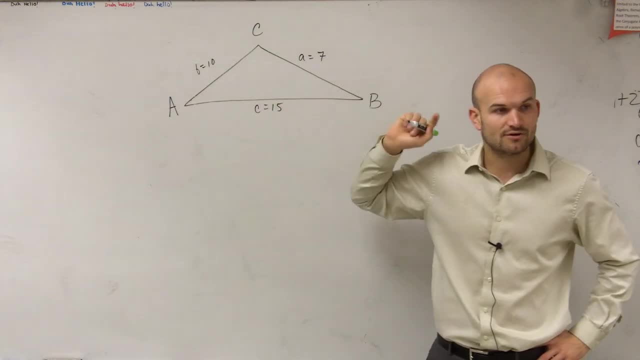 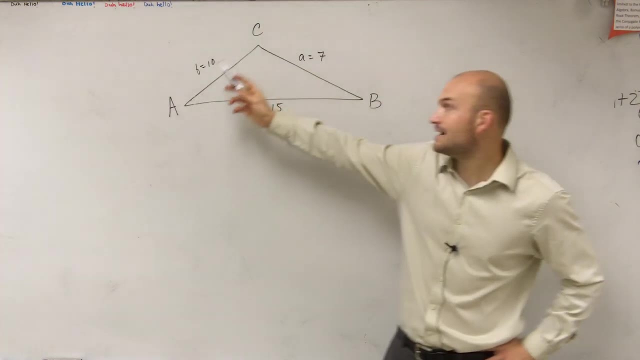 only angle. when I'm trying, when I have three side lengths, the angle that I want to solve for first is going to be the angle that is going to be potentially my largest angle. all right, so you can see, out of all these side lengths, here's 10. 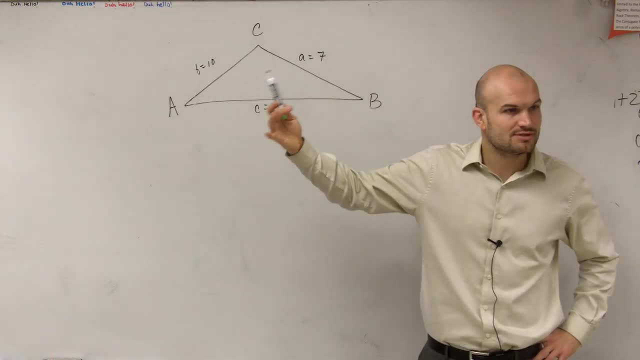 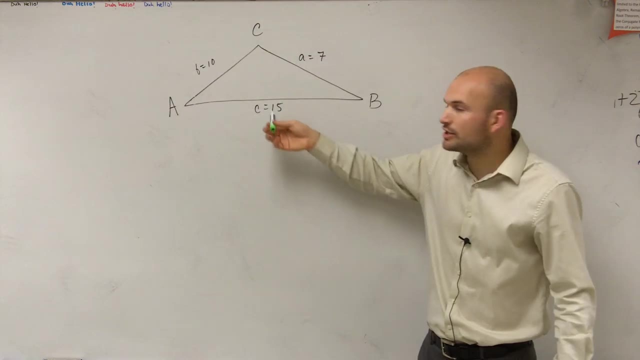 here's 7, here's 15. the angle that is potentially going to be the well, the angle that will be the largest is the one that obviously opens up to the largest side length. does that make sense? okay, so you're gonna want to find the angle C, and I'll explain why we're gonna find angle C first and why it's. 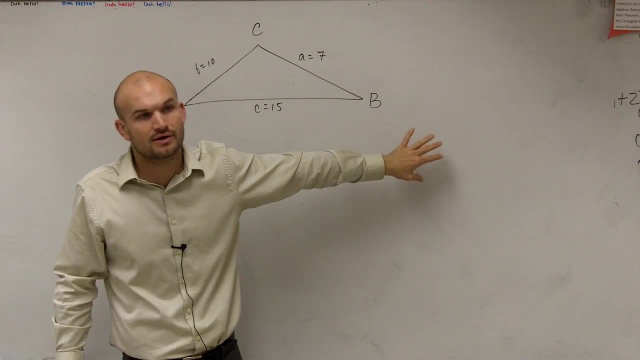 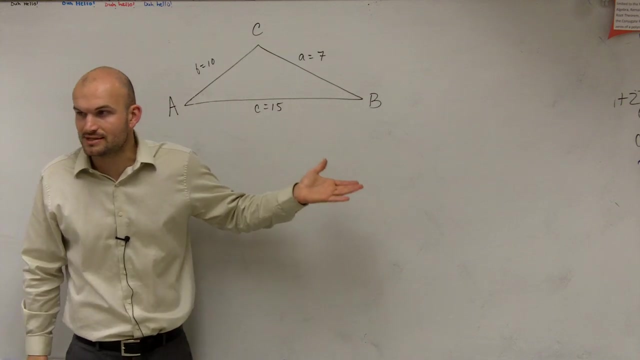 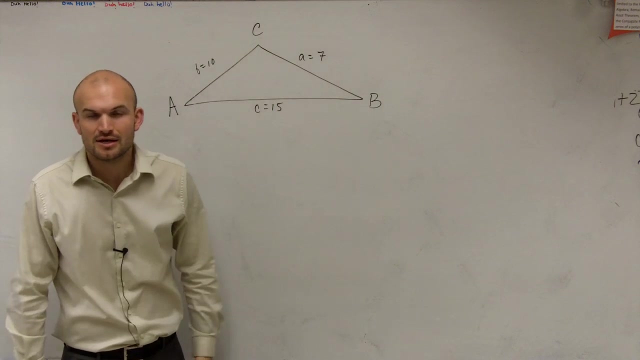 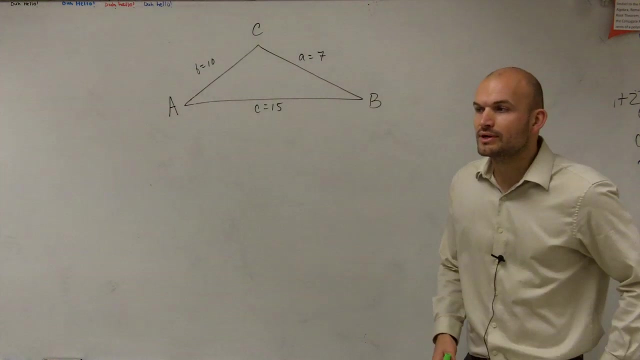 So we're given the side length of the opposing angle, of all three of the other angles right And their opposing side length, But we have a problem with this because we can't apply or use that proportion, because we don't even have a ratio that's complete right. You can't even set up a proportion that would have only one missing values because you don't have any of the angles. So to try to use this Kara for law of sines is not going to work alright. So what we're going to have to do is look into this by using the law of cosines. 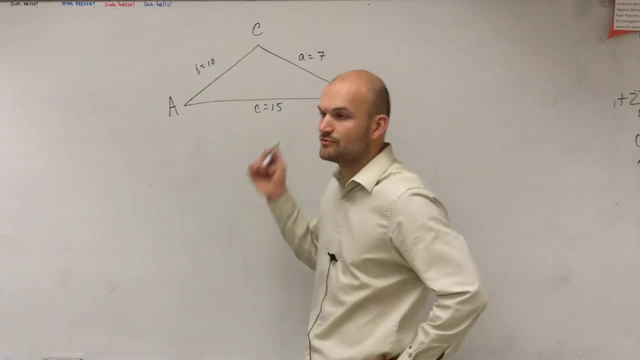 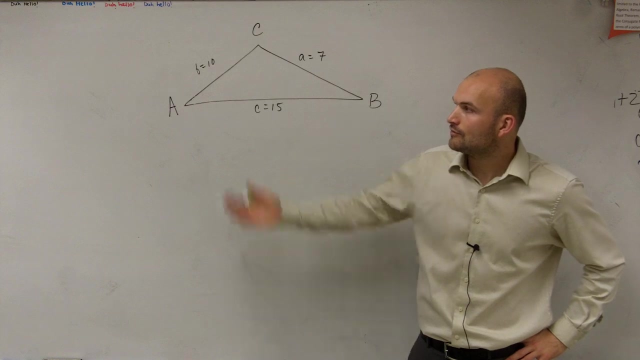 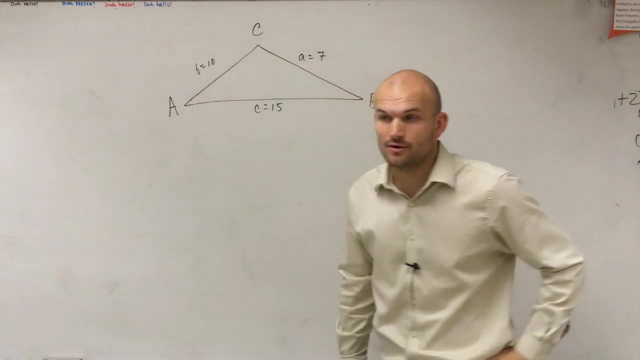 And there's a question here. There's a couple little tricks that we need to do in using the law of cosines, especially for a problem like this. You could say, well, I don't know what a, b and c are, And you can see, I wrote down the law of cosines over there. Well, for each one of those, they have a cosine of a, cosine of b or cosine of c. So you could say: well, you could just pick any one you want to and solve for that angle. 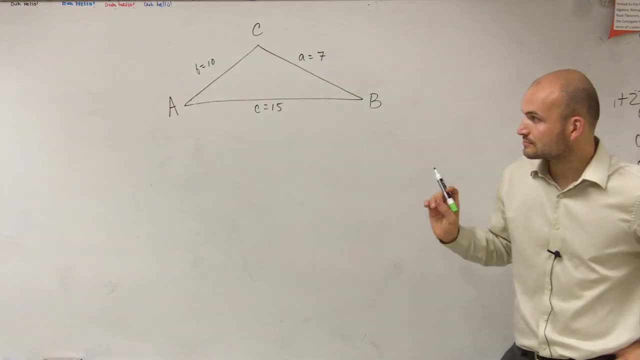 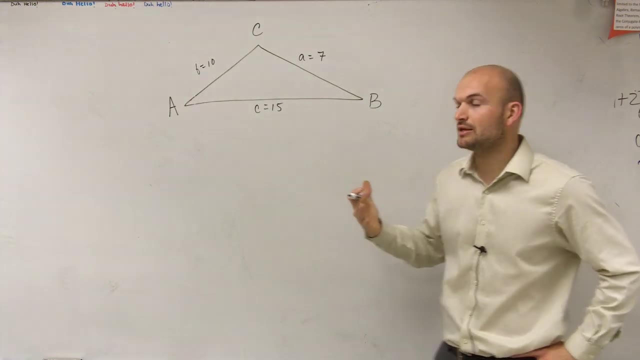 But the problem that we're going to want to come up with is, we don't want to arbitrarily just pick any angle. There's one angle that I want to be able to solve for first of all, And I'll kind of explain a little bit more about this later. 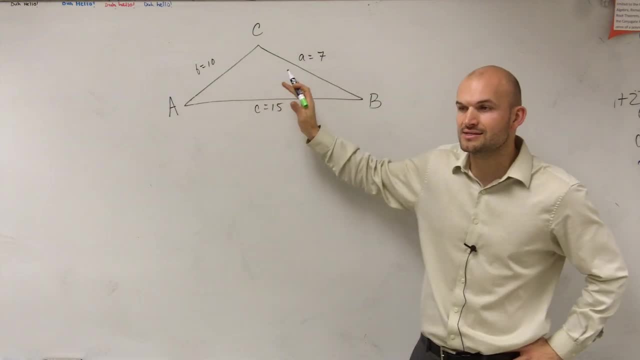 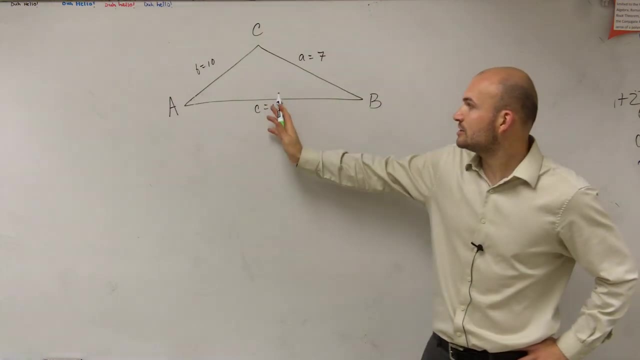 But the first angle, only angle. when I'm trying, when I have three side lengths, the angle that I want to solve for first is going to be the angle that is going to be potentially my largest angle. all right, so you can see, out of all these side lengths, here's 10. 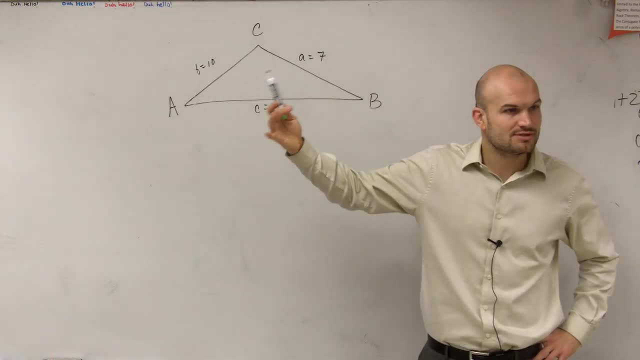 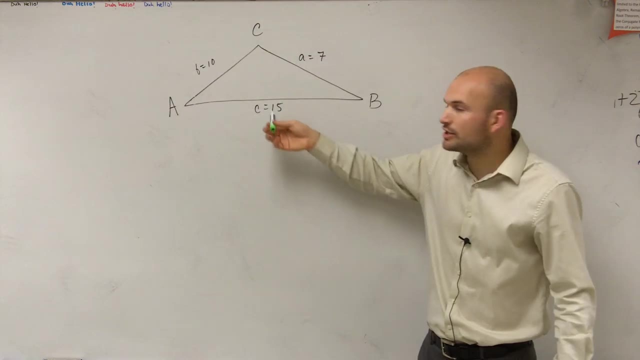 here's 7, here's 15. the angle that is potentially going to be the well, the angle that will be the largest is the one that obviously opens up to the largest side length. does that make sense? okay, so you're gonna want to find the angle C, and I'll explain why we're gonna find angle C first and why it's. 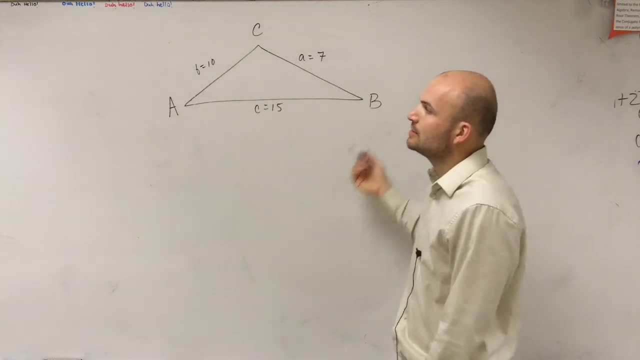 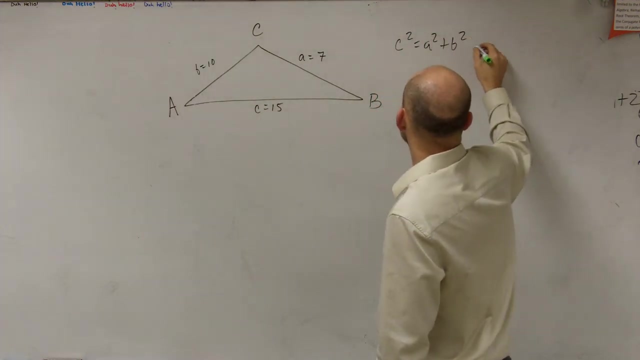 important to find angle C first, rather than finding angle A or angle B. so let's go and write in the formula for the log cosines for angle C. so we have: C squared equals a squared plus B squared minus 2 times a times B, times cosine of C, all. 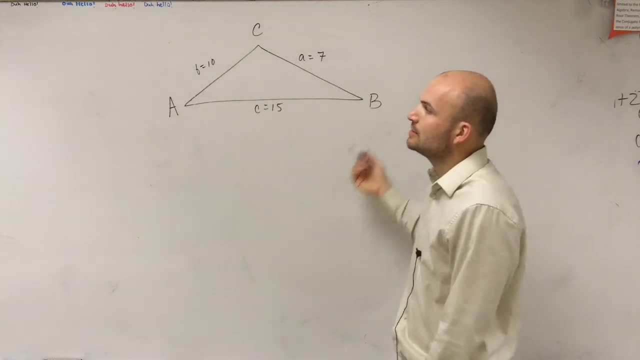 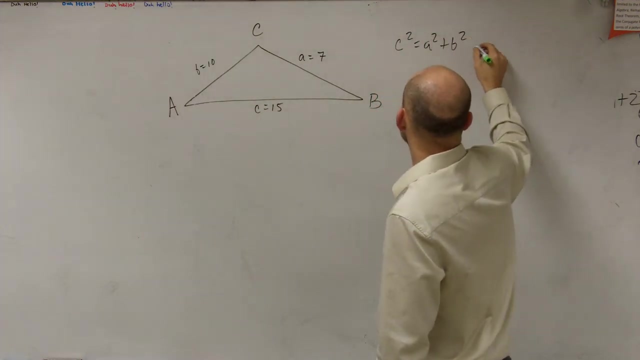 important to find angle C first, rather than finding angle A or angle B. so let's go and write in the formula for the log cosines for angle C. so we have: C squared equals a squared plus B squared minus 2 times a times B, times cosine of C, all. 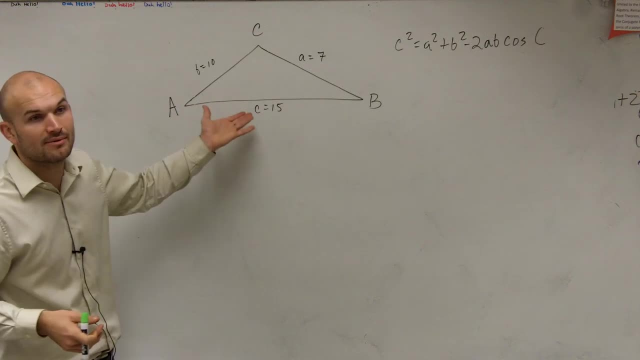 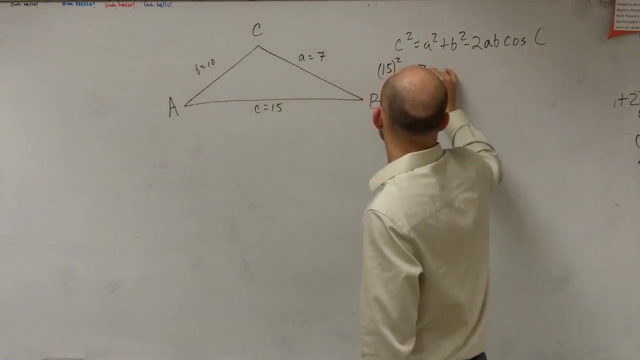 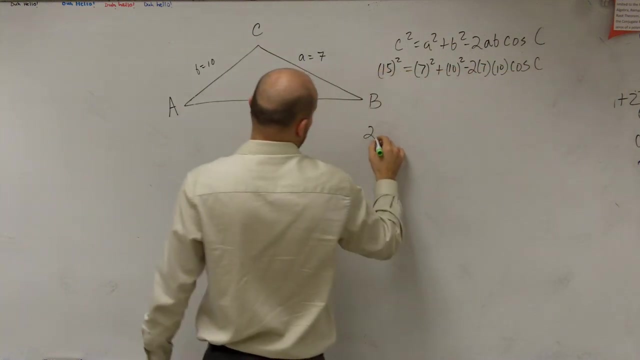 right. so now what we're going to do is just evaluate, plug in our values that we have and then solve. so we have C squared: 15 squared equals 7 squared plus B squared, which is 10 squared minus 2 times 7 times, 10 times the cosine of C. so 15 squared is gonna be 225, equals 49. 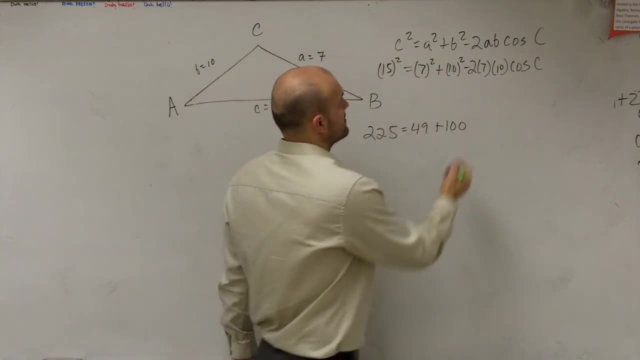 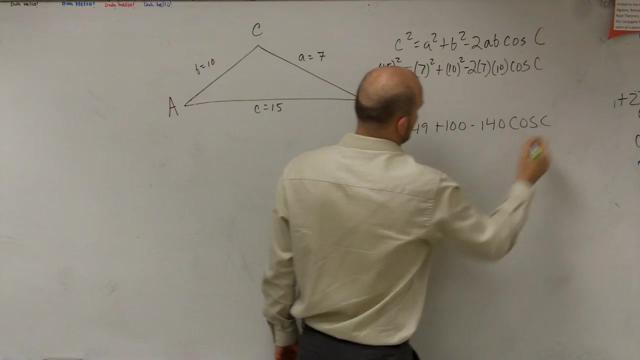 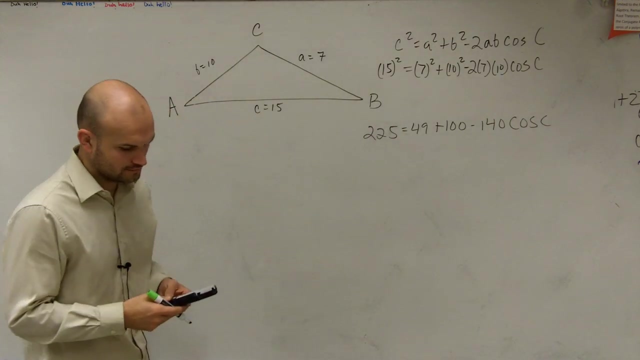 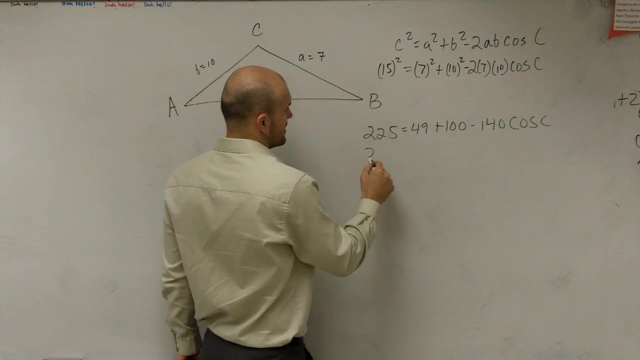 plus 100, and then we have 2 times 7, which is 14 times 100 is going to be a negative 140 cosine of C. everybody follow me so far, okay. so then what we're just going to look at is we can combine these like terms, so we have 225 equals 149 minus 140. 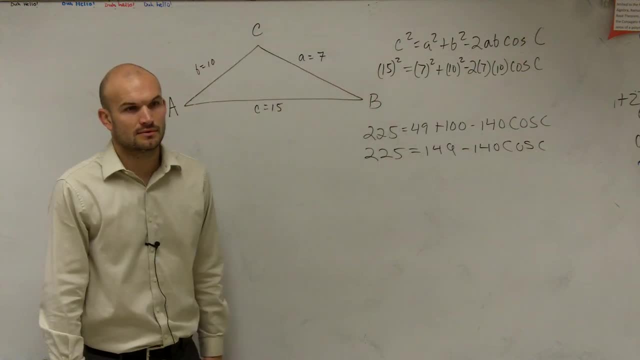 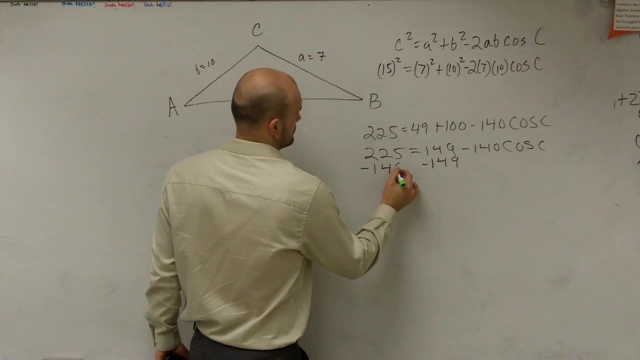 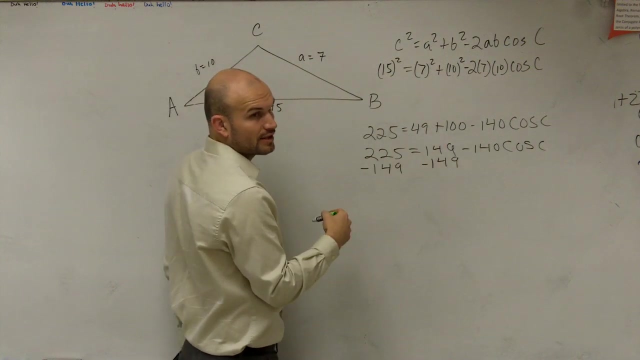 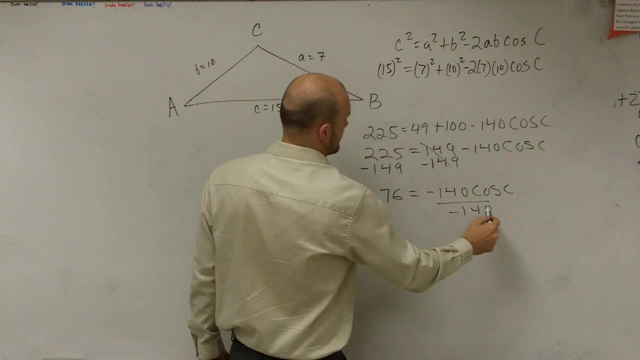 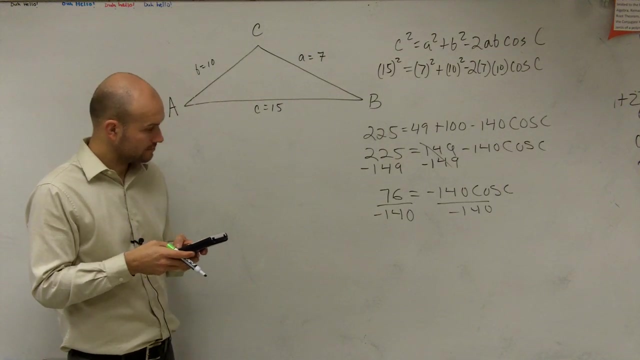 cosine of C. right, then we subtract, and sorry, well, no, I think you'll divide by negative 140, right, so this subtracts out the zero, and then this is going to leave us with 76. then we divide by negative 140. so there we say: divided by negative 140. so therefore I'm going to have negative. 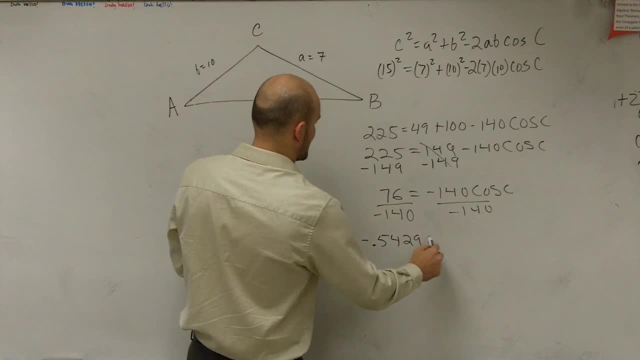 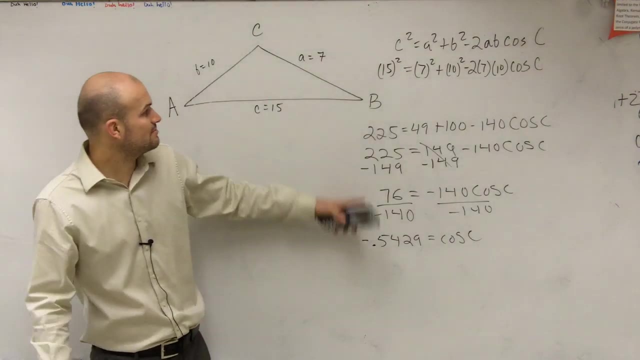 point five, four, two, nine equals the cosine of C. but remember, ladies and gentlemen, we're trying to find the angle C. this is going to be way too much of a small of an angle if we're looking into as far as this graph. that's a really. 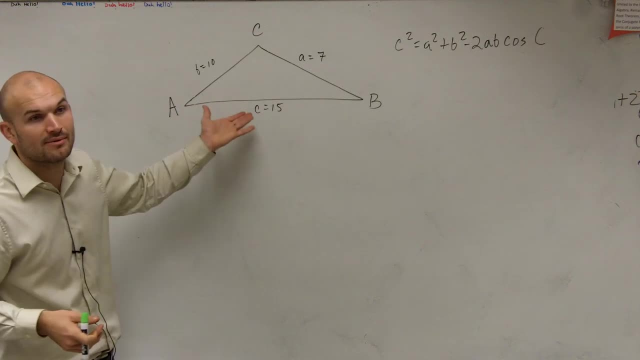 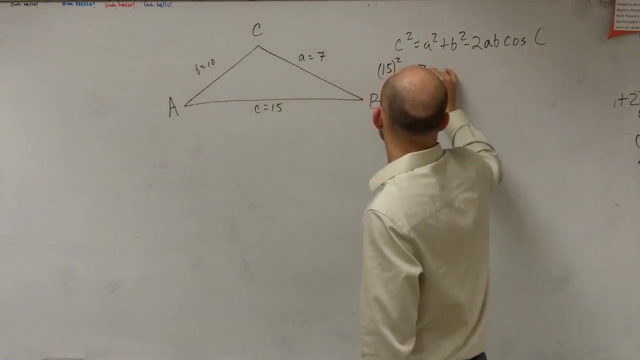 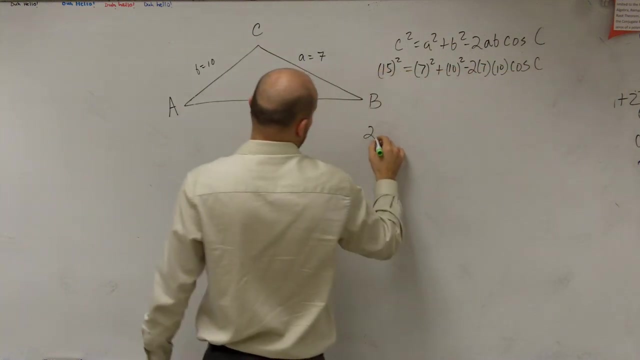 right. so now what we're going to do is just evaluate, plug in our values that we have and then solve. so we have C squared: 15 squared equals 7 squared plus B squared, which is 10 squared minus 2 times 7 times, 10 times the cosine of C. so 15 squared is gonna be 225, equals 49. 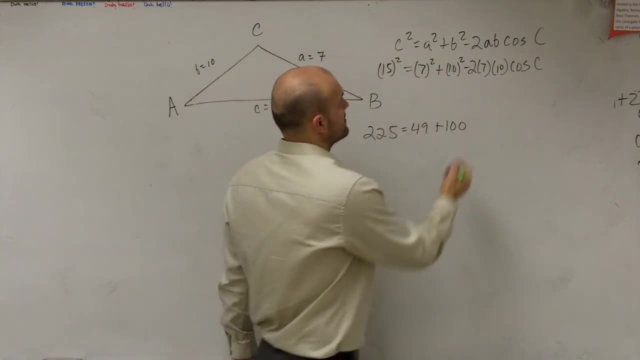 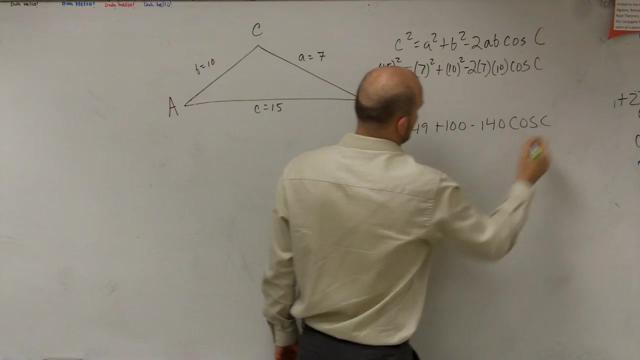 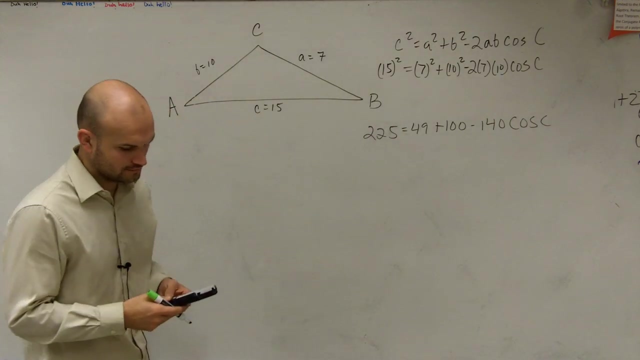 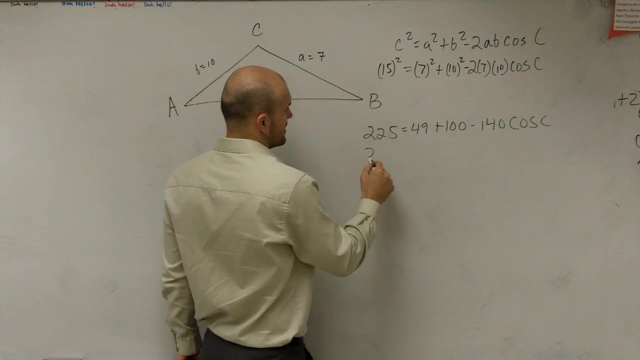 plus 100, and then we have 2 times 7, which is 14 times 100 is going to be a negative 140 cosine of C. everybody follow me so far, okay. so then what we're just going to look at is we can combine these like terms, so we have 225 equals 149 minus 140. 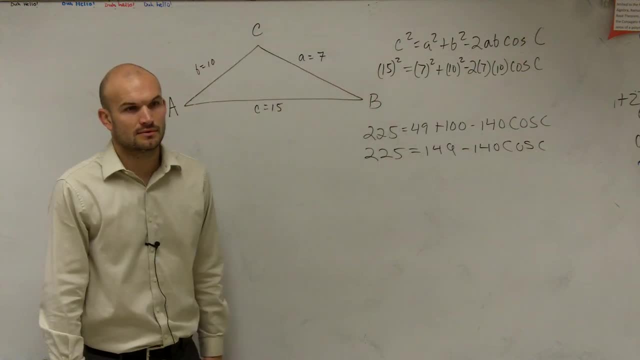 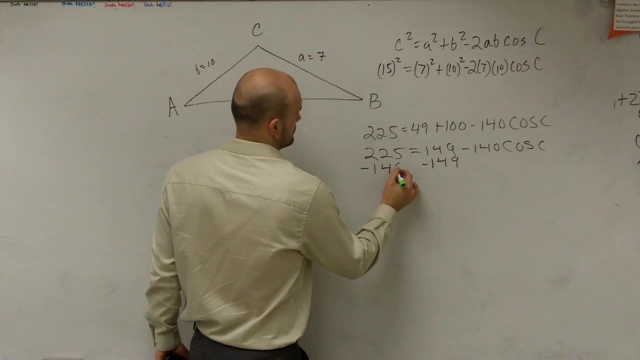 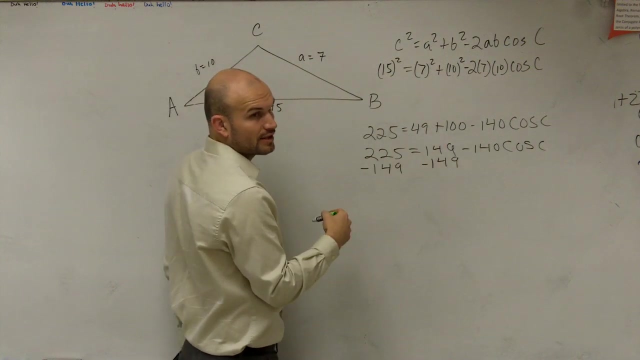 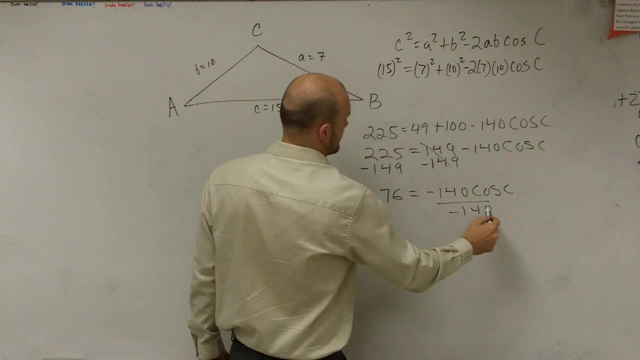 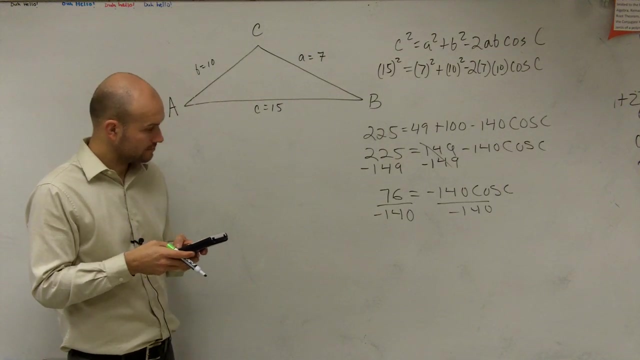 cosine of C. right, then we subtract, and sorry, well, no, I think you'll divide by negative 140, right, so this subtracts out the zero, and then this is going to leave us with 76. then we divide by negative 140. so there we say: divided by negative 140. so therefore I'm going to have negative. 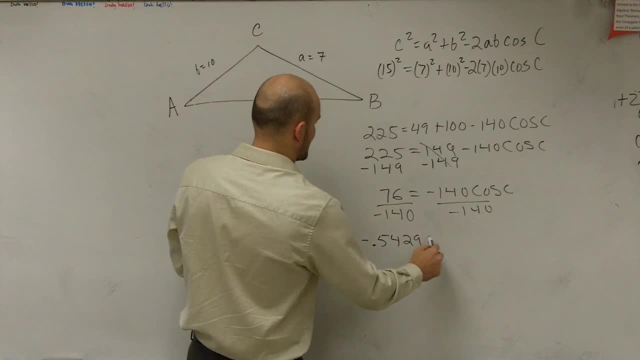 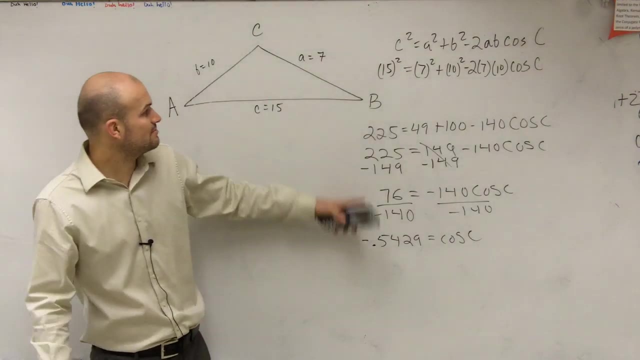 point five, four, two, nine equals the cosine of C. but remember, ladies and gentlemen, we're trying to find the angle C. this is going to be way too much of a small of an angle if we're looking into as far as this graph. that's a really. 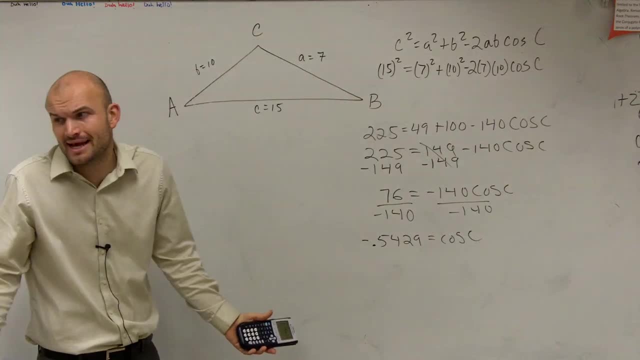 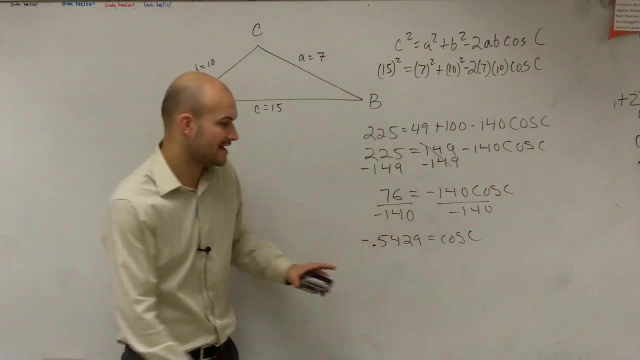 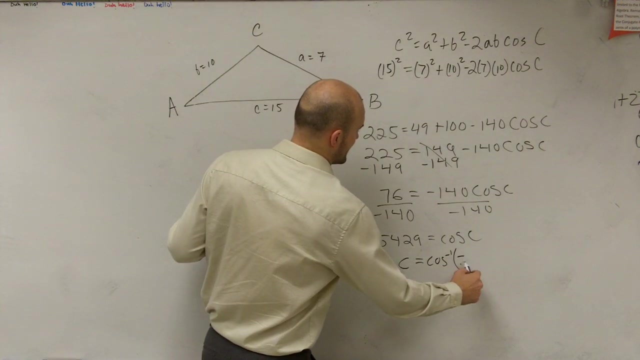 really small, cute angle, right, and we said it has to be the smallest angle or the largest angle. so that's not gonna make sense. remember, to find the angle C it says cosine of my angle C equals this value. so to find the value of C I'm now going to have to use inverse cosine of negative. point five: 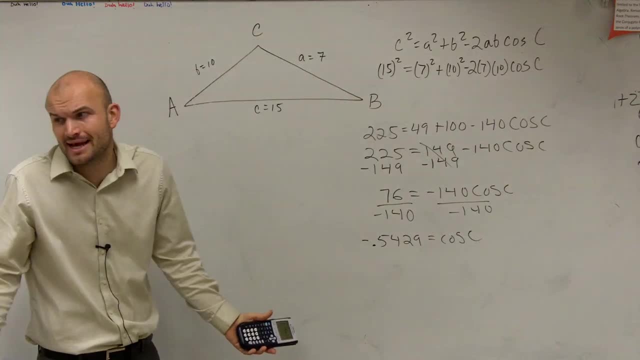 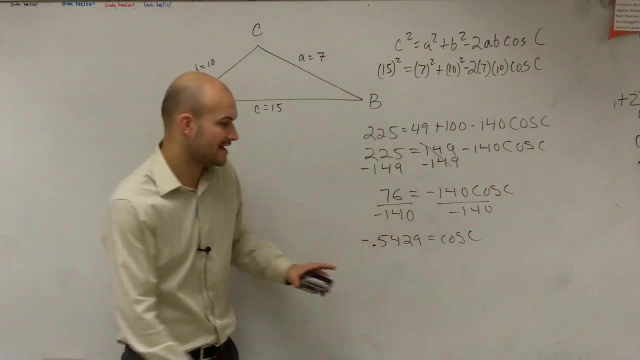 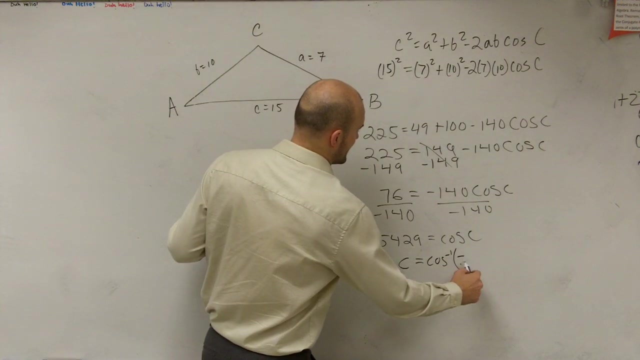 really small, cute angle, right, and we said it has to be the smallest angle or the largest angle. so that's not gonna make sense. remember, to find the angle C it says cosine of my angle C equals this value. so to find the value of C I'm now going to have to use inverse cosine of negative. point five: 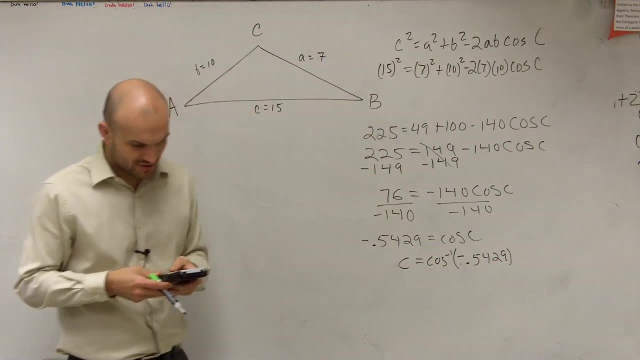 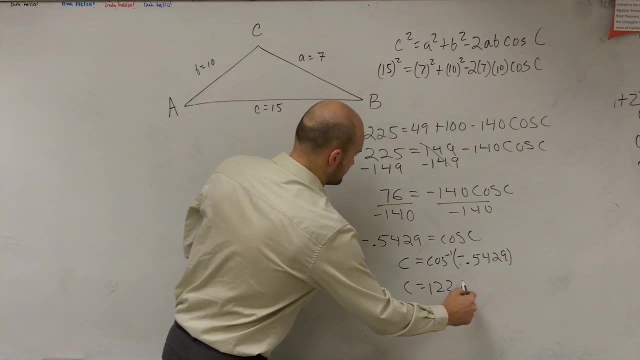 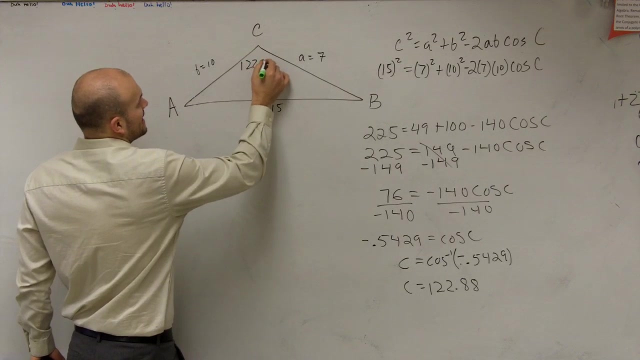 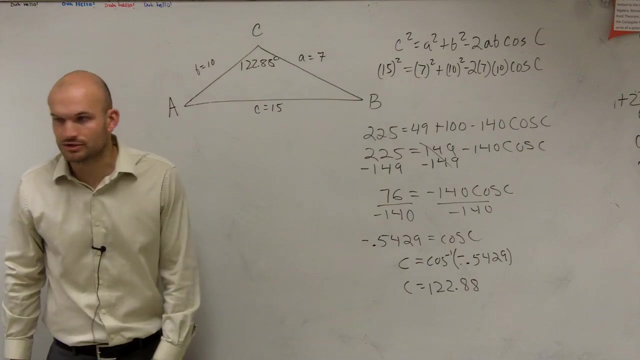 four, two, nine. so I do inverse cosine. second answer: and I get: C equals 122 point eight, eight. so I could. C equals one hundred twenty two point eight, eight degrees. okay, so why is that so important for us to be able to do this? well, now for the remaining. 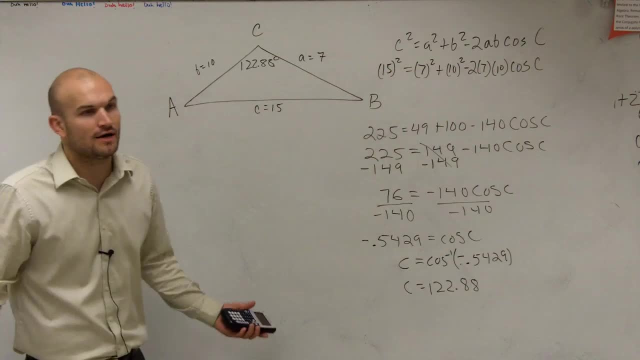 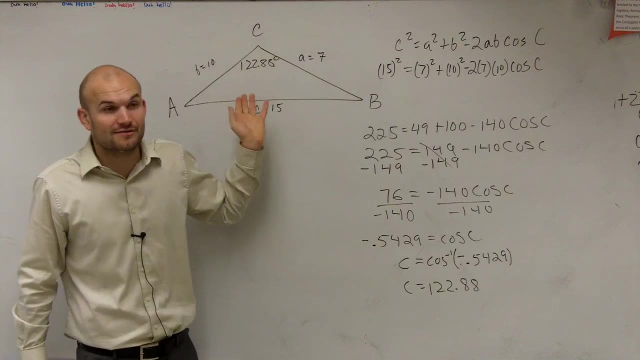 sides to find our remaining angles. now we're going to have to do is apply the law of law of sines, right and the important thing about noticing this as remember when we applied the law of sines. we're gonna have to evaluate, but we're going to use again. 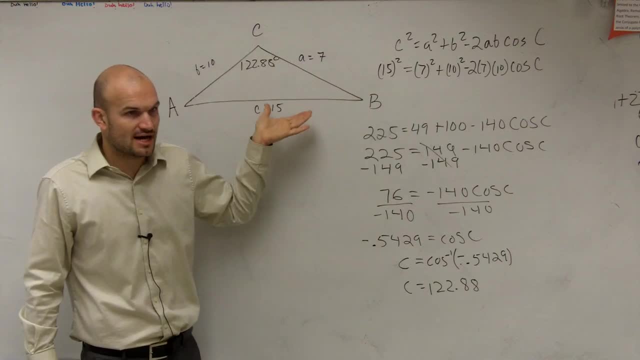 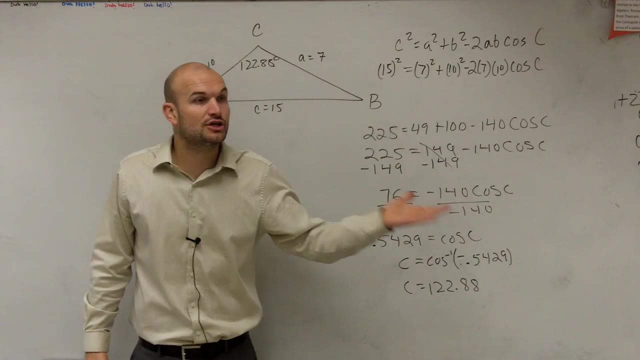 the inverse sign right, we're going to have to use the inverse sign to find the to define one of these angles. and remember, using the inverse sign, we had to determine was it acute or was, or did we use the obtuse angle right? remember, when we had the ambiguous case we had that you know those possible two. 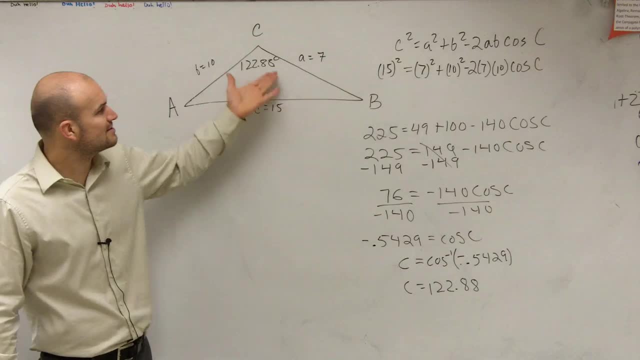 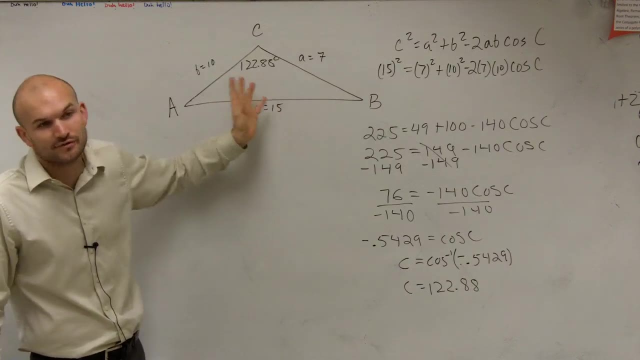 different solutions and what we always determine was: since we're figuring out this value, we know that these other two angles have to be acute, so you don't even need to worry about even though we have three sides. it's not a it's not a side-side angle, but it's important for you guys to understand now that I have 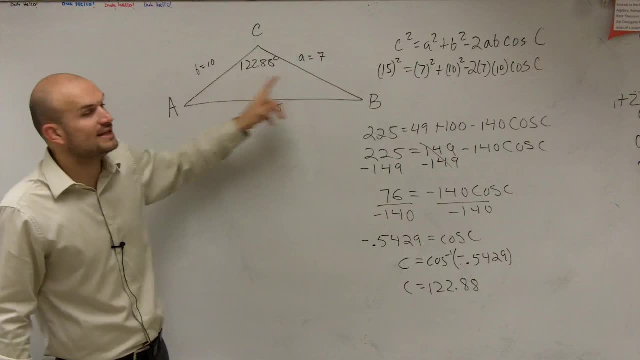 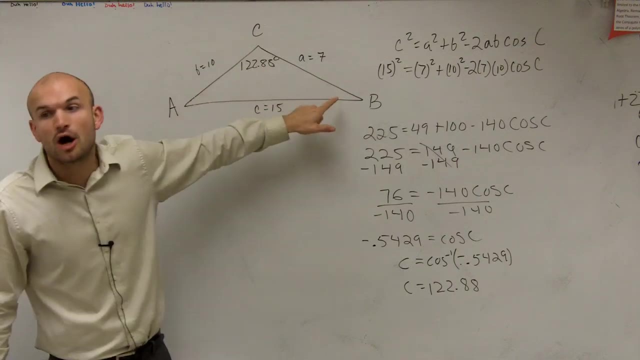 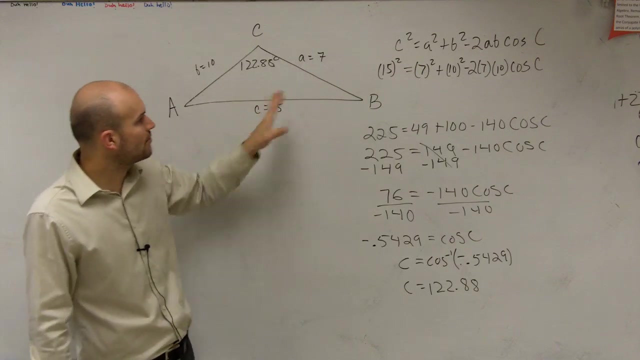 an obtuse angle. now that I found the largest angle, I know that these two angles are acute. all right. or even if this was acute, you still know that these other two angles also have to be acute, because this is the largest angle out of the three. okay, so it's just important to always find the largest angle first. 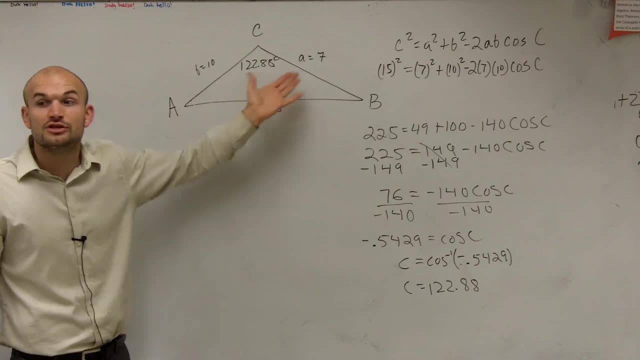 because then you know that your other two angles are always going to be acute. it's much easier to do that than to say, oh, I found an acute angle, the other two- one could be obtuse, one could be acute. it gets a little dicey working, it that? 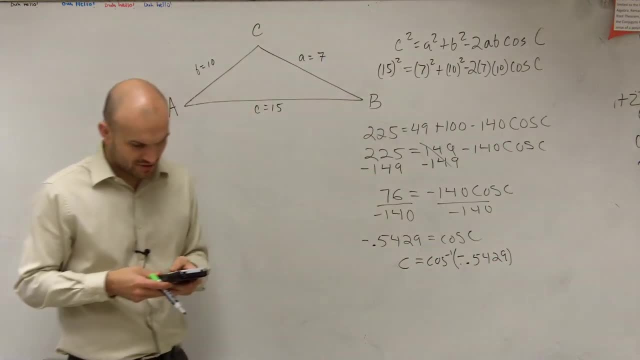 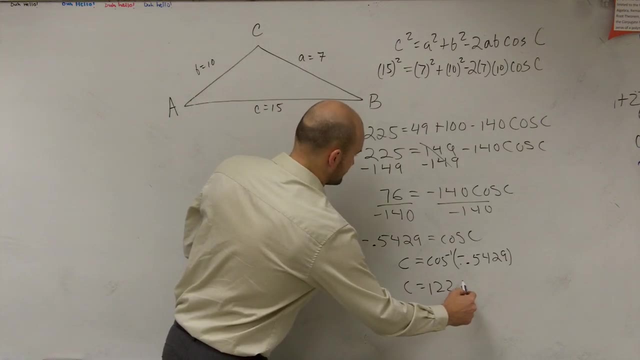 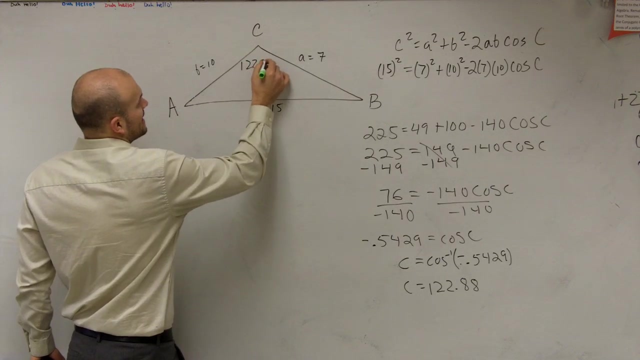 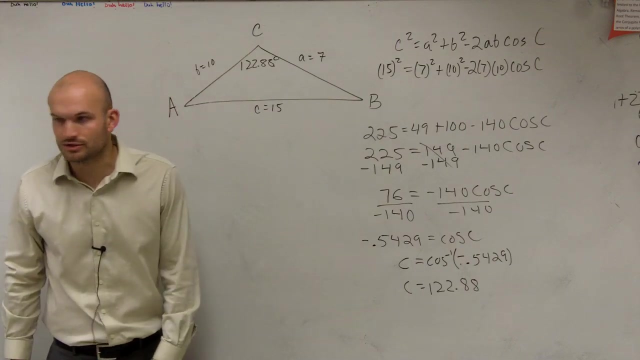 four, two, nine, so I do inverse cosine. second answer: and I get C equals 122, point eight, eight. so I could see equals 122.88 degrees. ok, so why is that so important for us to be able to do this? well, now for the remaining sides to find our remaining angles. now we're going to have 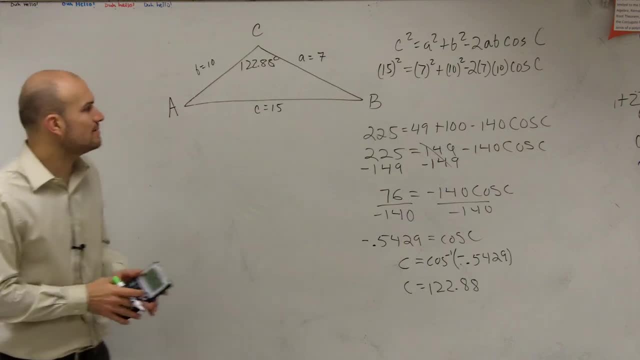 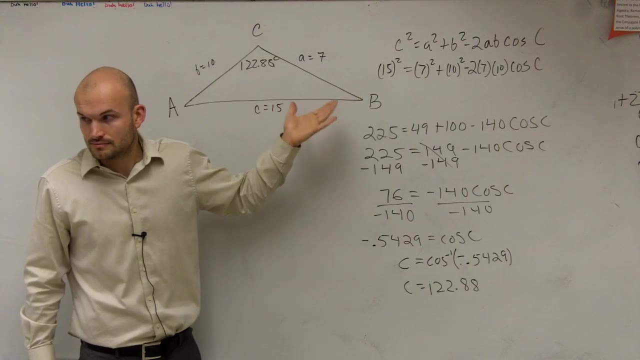 to do is apply the law of law of signs right- and the important thing about noticing this is my boy. when we applied the law of signs, we're gonna have to evaluate, for we're gonna have to use again inverse side right. we have to use the inverse sign to find. 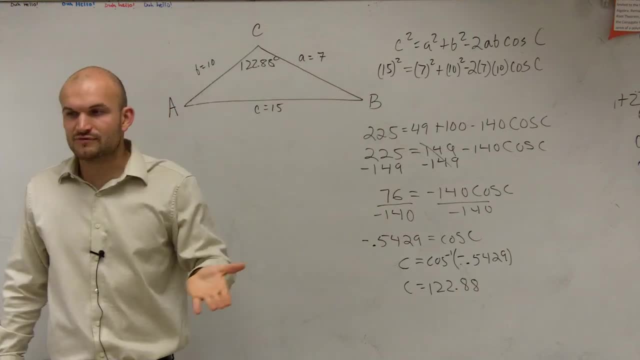 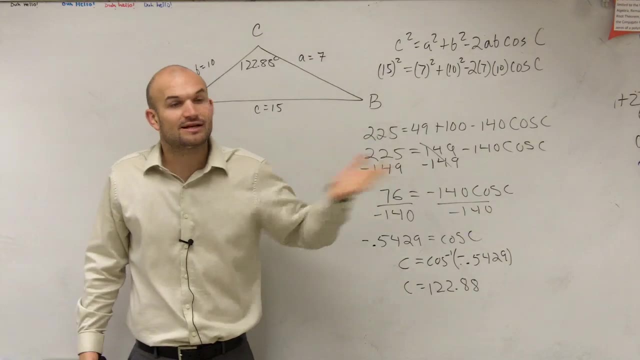 to define one of these angles and remember, using the inverse sign, we had to determine: was it acute or was, or did we use the obtuse angle right? remember, when we had the ambiguous case, we had that you know those possible two different solutions and what we always determine was: since we're figuring out, 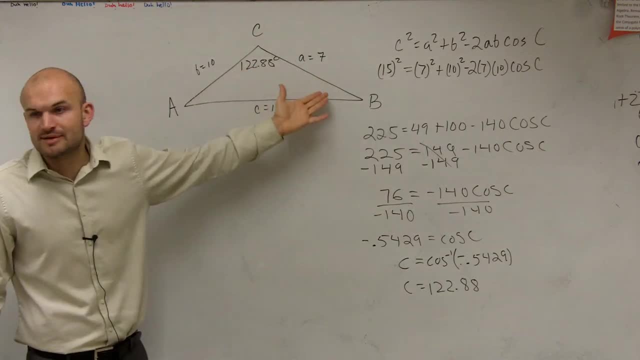 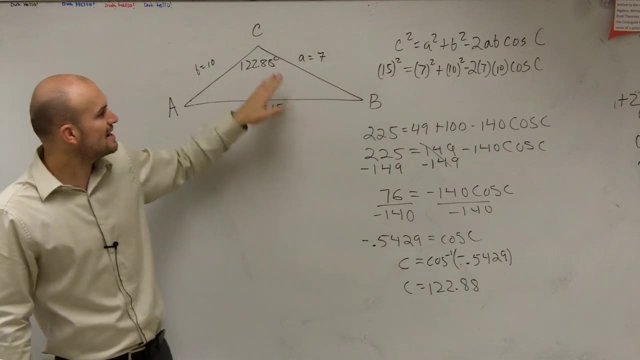 this value. we know that these other two angles have to be acute, so you don't even need to worry about even though we have three sides. it's not a. it's not a side-side angle, but it's important if you guys understand now that I have an. 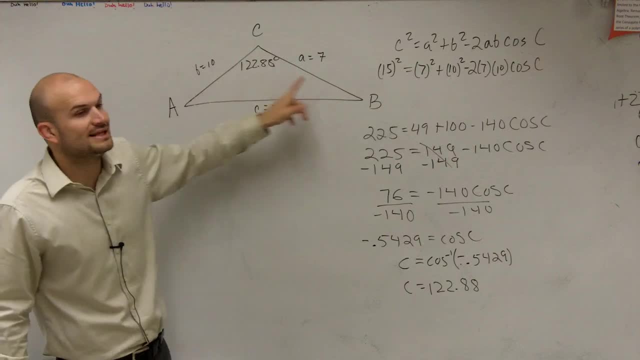 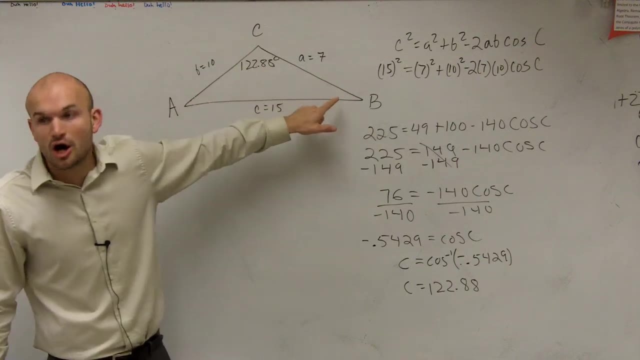 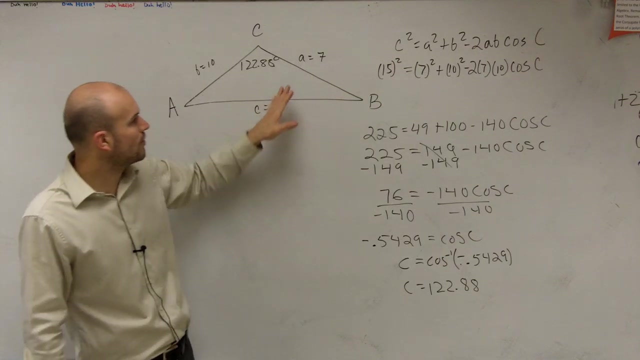 obtuse angle. now that I found the largest angle, I know that these two angles are acute. all right. or even if this was acute, you still know that these other two angles also have to be acute, because this is the largest angle out of the three. okay, so it's just important to always find the largest angle first. 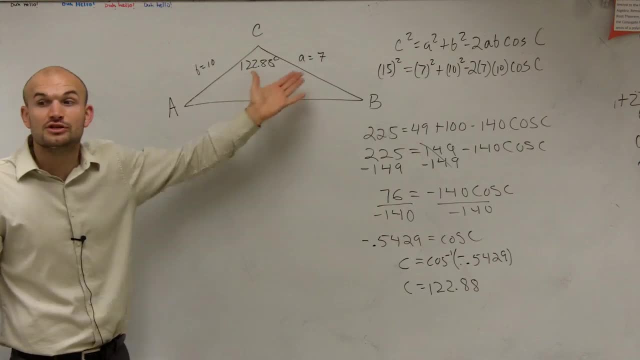 because then you know that your other two angles are always going to be acute. it's much easier to do that than to say, oh, I found an acute angle, the other two- one could be obtuse, one could be acute. it gets a little dicey working, it that? 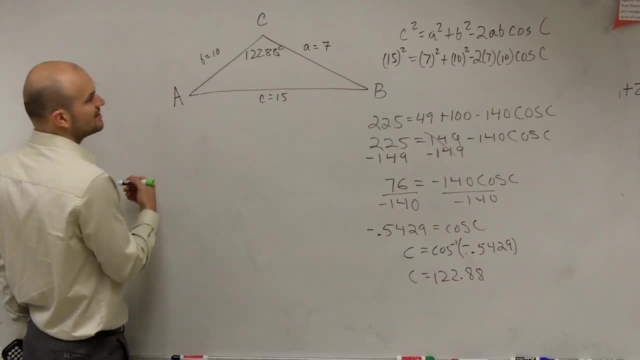 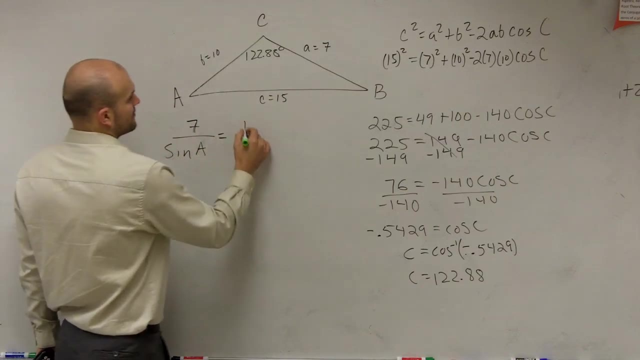 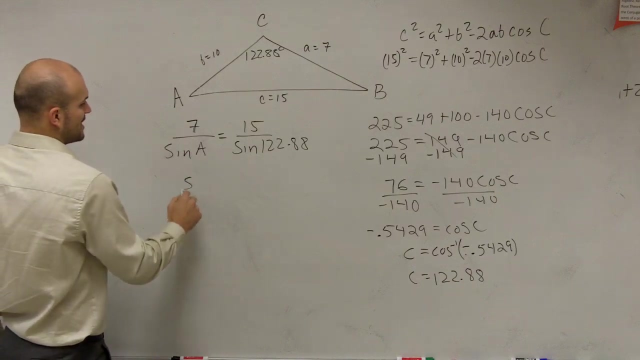 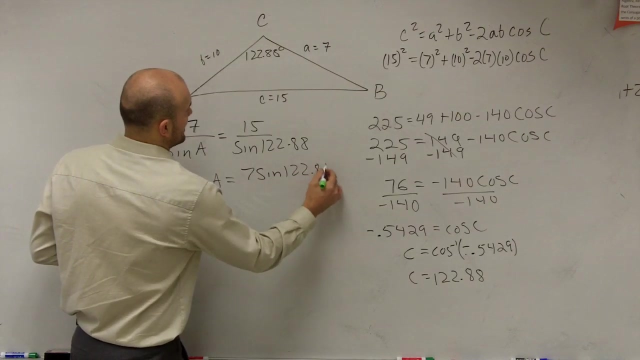 way. so now to find angle a or b we can just use the law of sines. I'll do a. so 7 over sine of a equals 15 over the sine of 122.88. so by solving for sine of a, sine of a equals, we could do 7 times sine of 122.88 divided by 15.